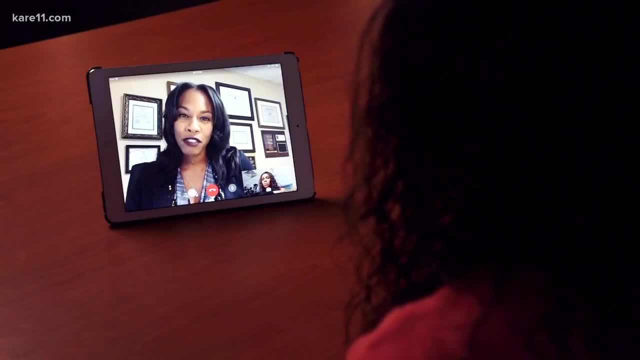 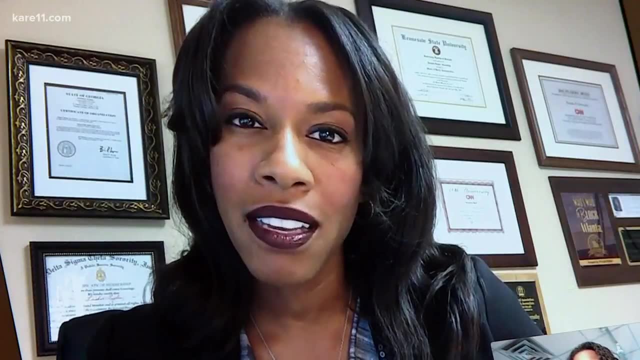 I could. It was a city that raised me, a city that I love, a city that also took my father's life. He was shot as well by teenagers there ages 15,, 19, and 21, when I was just five years old. 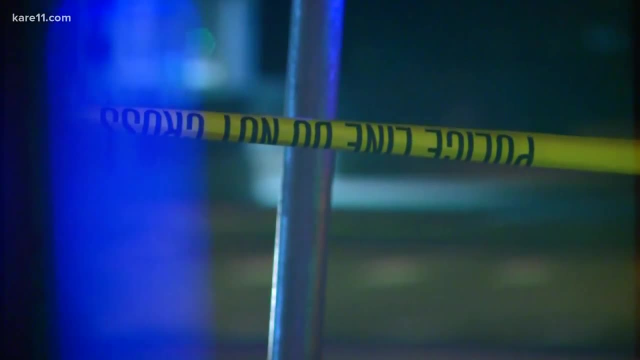 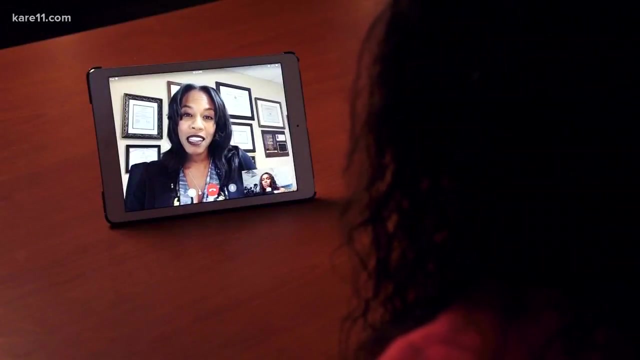 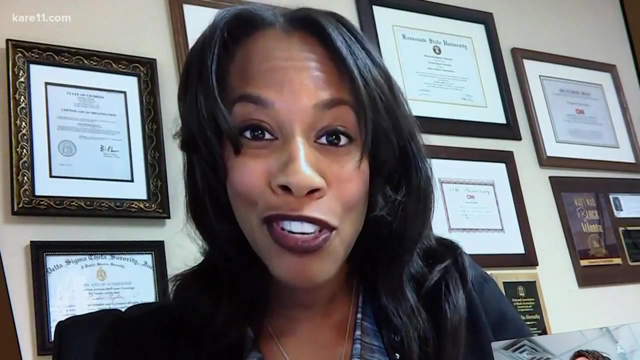 Bell says teens like the ones who killed her father were the inspiration behind a scholarship foundation bearing her dad's name. We provide scholarships, mentorships and life skills seminars to young men who are middle class, Sometimes fall through the gaps. You know they may be the C student and oftentimes they don't. 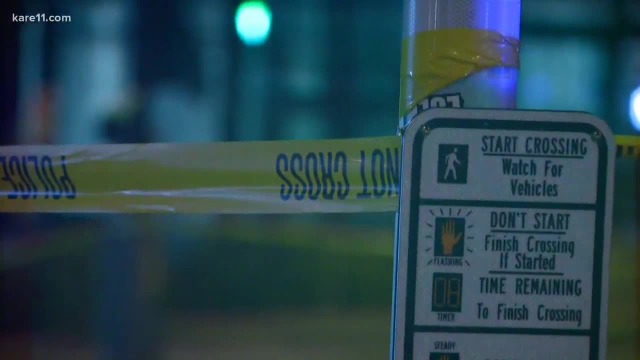 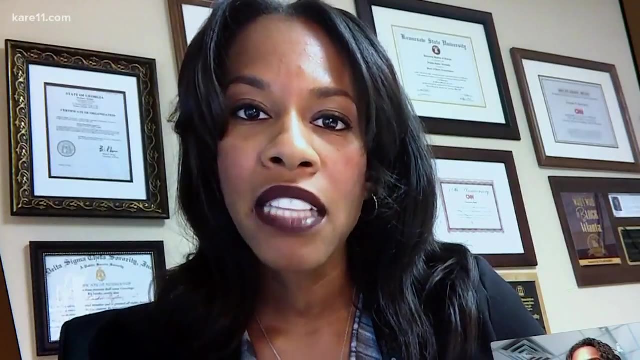 have opportunities or resources to them. Mentoring addresses the topic some ignore. You don't see these killings in mass numbers like this in other races. You know, how can we expect someone else to respect us if we don't respect ourselves? So the Black-on-Black crime that is. 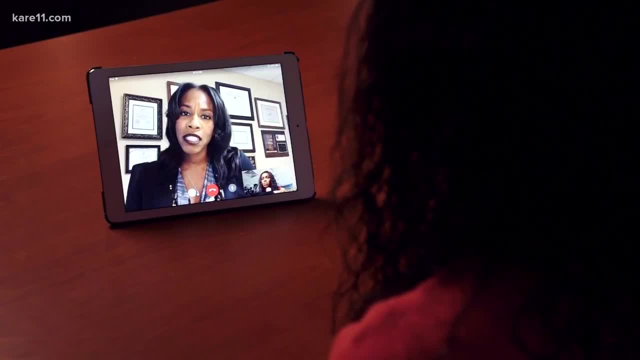 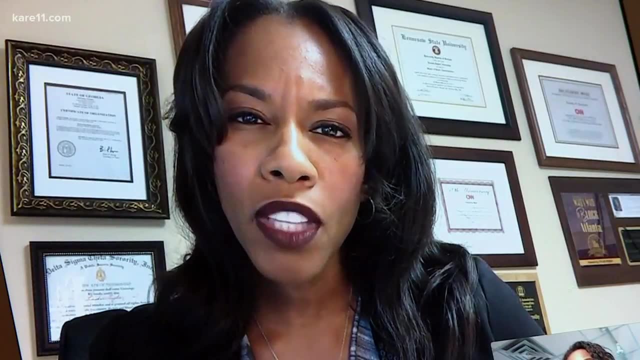 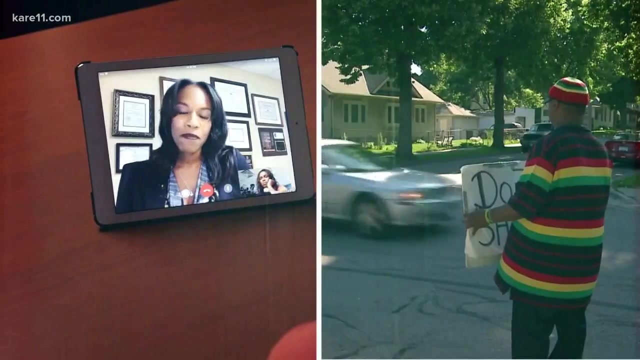 plaguing not only Chicago, Detroit, Minneapolis, so many cities across the nation. but you have to start at home. You have to take care of home, You know. you have to make sure that young people respect our race From her office in Atlanta to street corners in Minneapolis, both Bell and Wilson. 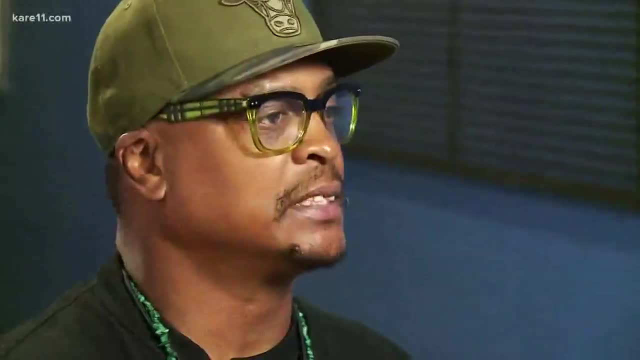 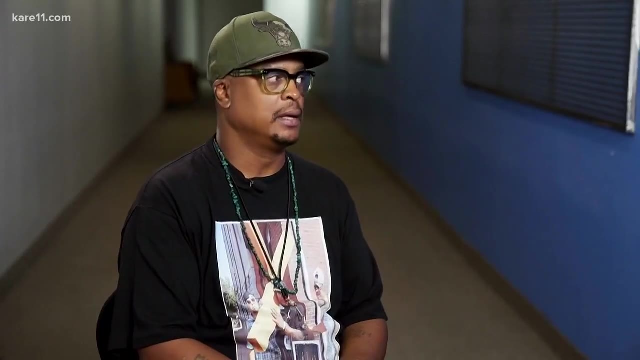 Chicago natives are doing their part. If I have to stand by myself in front of a firing squad, I'm going to be that one who let the youth in the community know that this is right. We can't be quiet about it anymore. 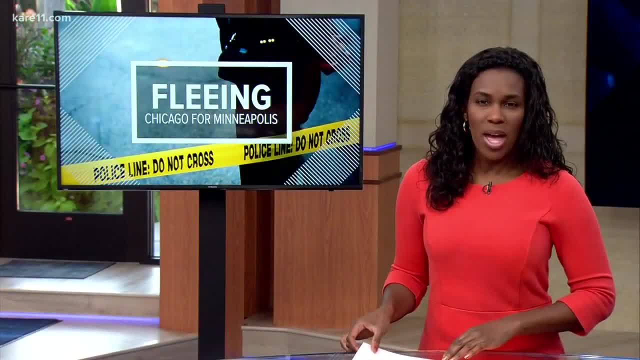 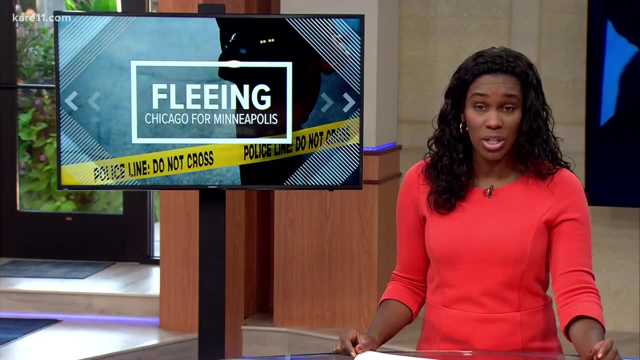 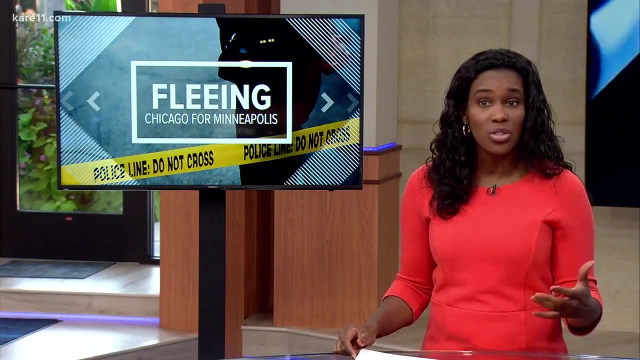 According to the FBI's Uniform Crime Reporting data for 2016,, 90.1% of Black victims of homicide were killed by other Blacks. But the story doesn't stop there: 83.5% of whites were killed by other whites. Some will argue: this data shows this is a truth. 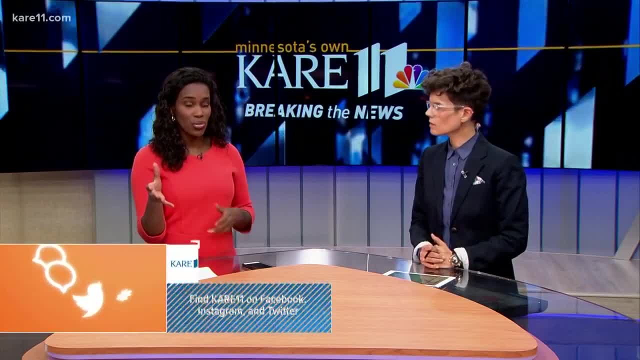 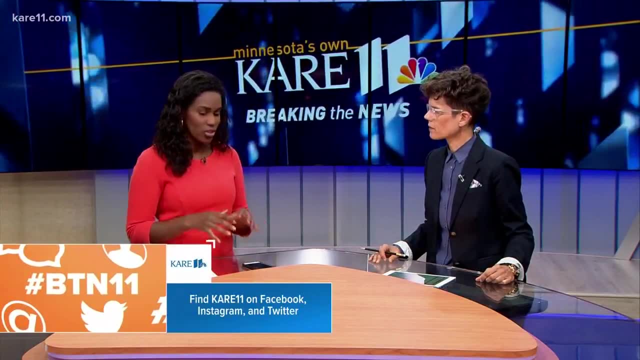 across racial boundaries. Tanisha, who you just heard from in this story, worked as an executive producer for CNN for 13 years and she simply said it was haunting her as she would write those stories about gun violence in Chicago, And it seems to be a problem that. 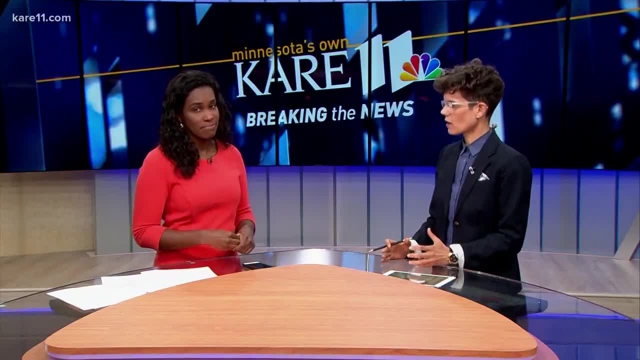 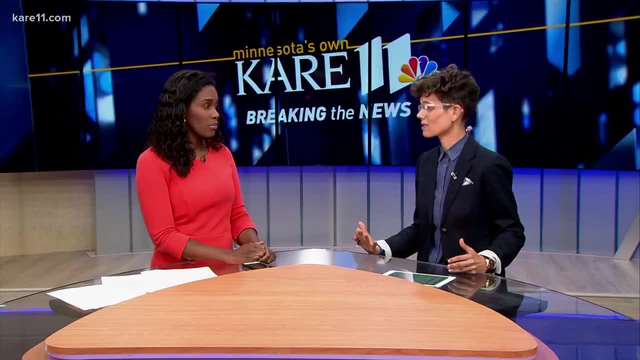 is just not going away because we see holiday weekend reports out of Chicago: 60,, 70,, 80. It's unfathomable and my heart breaks, but it certainly goes out to those people who are doing the work on the streets. That's incredible stuff. Yeah, they're in the trenches. Yeah, absolutely. Thanks, Adrienne.